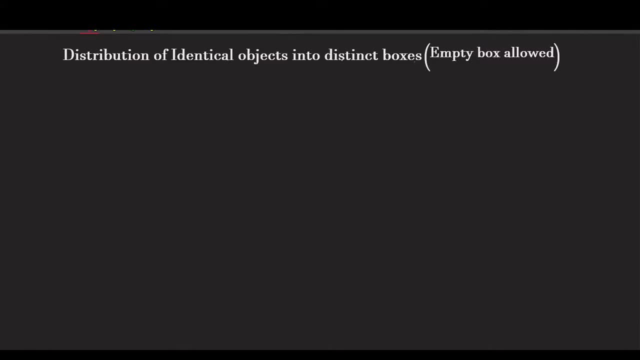 So hello students and friends. So here in this class we are going to discuss a concept of permutations and combinations, that is, distribution of identical objects into distinct boxes. So in the previous class of my permutation combinations playlist I discussed about division of the different objects into groups, But here we will discuss distribution of identical objects. How to distribute identical objects. 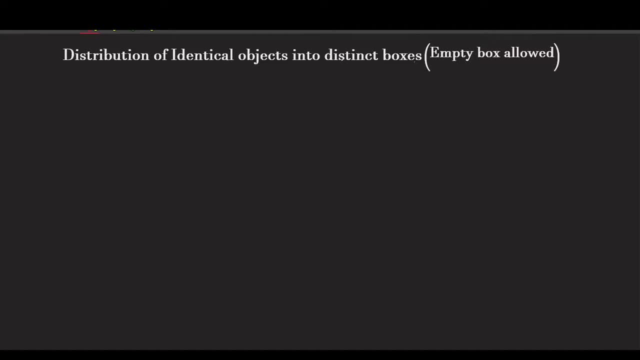 How to distribute identical objects into different boxes. Let's say you have n identical objects. Let's suppose you have n identical objects And we want to distribute these n identical objects into r different boxes. We want to distribute into r different boxes. So what is the answer for this? How many ways, The number of ways we have to find out The distribution, the number of ways of distributing the n identical objects into r different boxes. Now let's see, with some examples, I will explain how to get the rule or formula for finding this number of distributions. Let's say, if I take n value, let's say simply, I will take 6 and I will take r is equals to 3.. So what is n? 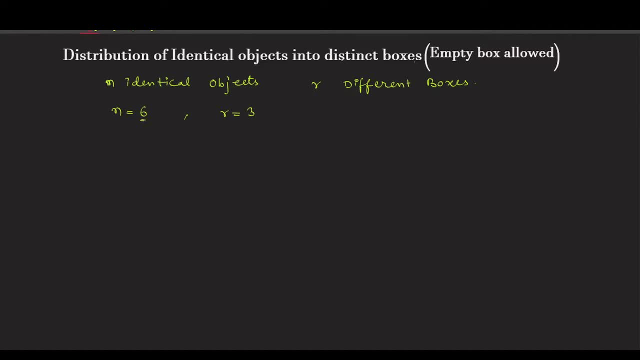 What does it mean? The question is like this: How many ways you can distribute 6 identical objects into 3 different boxes? So if you have 3 different boxes and you have n identical objects, how many ways you can distribute them? So let's say you have 3 different boxes here. They all are different. If you want, you can name them. Say this is x box and this is y and this is z. If you want, you can give the names for them. 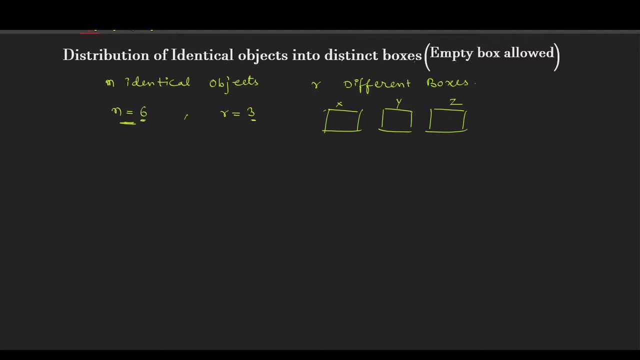 Keep these 6 identical objects into 3 boxes. One of the ways you can write like this. One of the ways you can keep 2 identical objects here and 3 here and 1 here. So what is the meaning of this? indirectly, In the box x you are keeping 2 identical objects and in box y you are keeping 3 and in box z you are keeping 1 object only. So means x value 2, y value 3 and z value 1.. 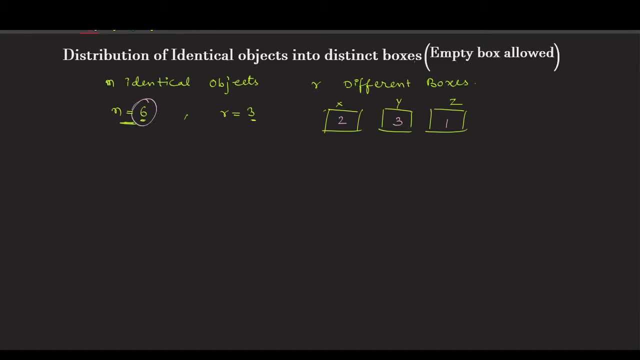 So what we are expecting to find is these 6 identical objects. Let's say I call u, u, u, u, u and u. So here we have 6 identical u's Means say they are identical objects and you want to place these into 3 boxes. So whenever you want to keep these 6 identical balls into 3 boxes, you need to divide this into 3 groups. Then you can put those identical objects into that x box. 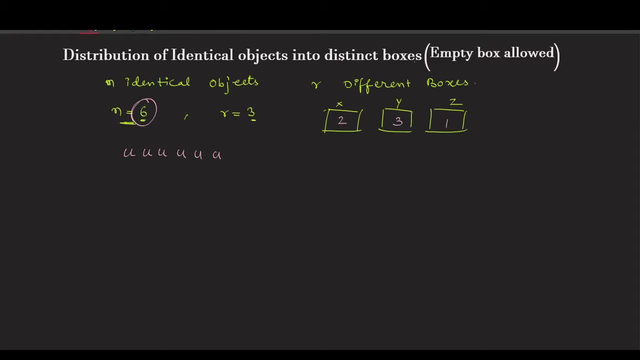 So to break this into 3 groups, how many separation symbols I need? For example, if I take a separation symbol here and one more separation symbol is here, then you can say: the first box will be having 2 identical and the second box will be having 2 and the third box also will have 2 identical. 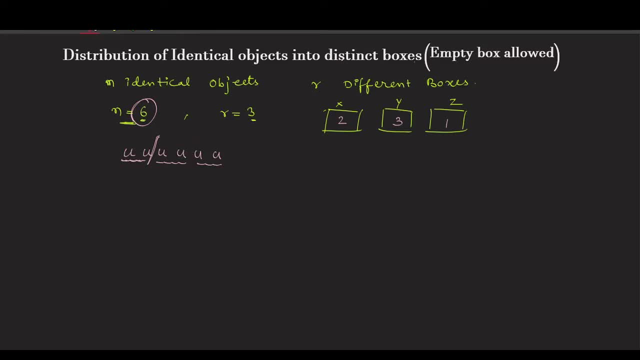 Instead of these two separation symbols, let us say I will take the separation symbol somewhere else. Say, here I took one separation symbol and here I took one separation symbol. So before the first separation symbol, how many identical objects you are seeing? 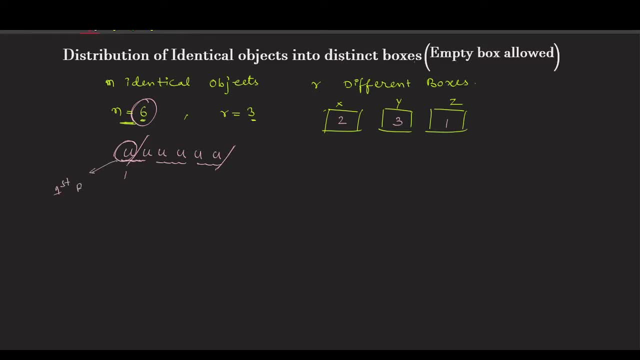 That will go to the first box. That will go to the first box And how many you are seeing between these two separation symbols? Five. So these will go to second box And then the remaining means after the second separation symbol. how many are there here? 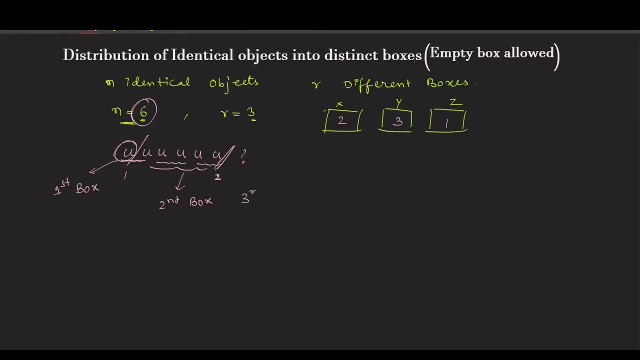 Zero, So that zero will go to third box. I hope you understood. So what is the meaning of this? If you keep two separation symbols in these, among these six identical objects, you will get one way of the distribution. So indirectly, let us say, I have six u's and two s. 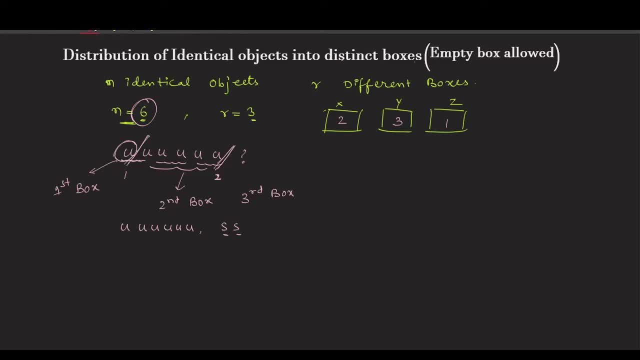 I call these two s as separation. Instead of taking these lines, I am supposing now s and s. Now let us see this here. Let us see one arrangement of these six identical and two s. How many ways you can arrange them means totally. we have eight objects here. 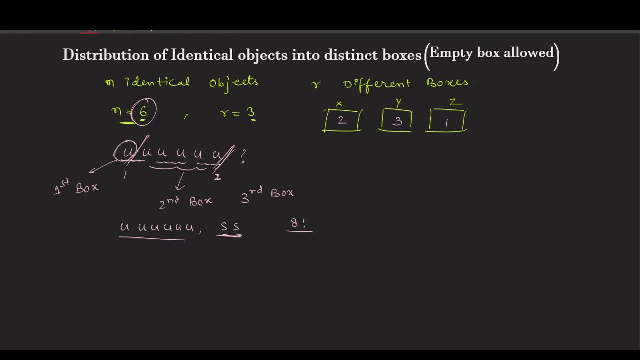 So it can be arranged. in how many ways? Eight factorial by six u's are there, so six factorial and two s are there, so therefore two factorial. So how many ways you can arrange these six letters, u letters and two s letters, right? 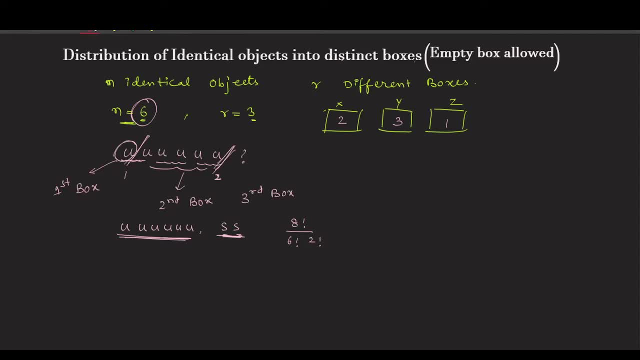 in a row Is what? Eight factorial by six, factorial by two factorial. Now why I am finding the arrangements. Now let us see one arrangement: U s u s u u u? u. so what is the meaning of this? 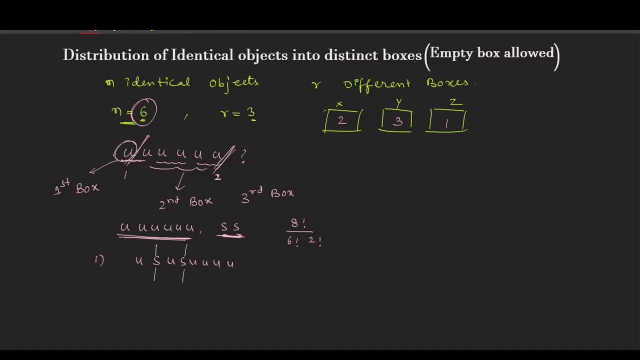 This is the separation symbol. here you have Second separation symbol. here you have Now before Before separation symbol. how many objects you are seeing? One? This will go to the first box Right. This will go to first box And in between, two separation symbols. how many are there? 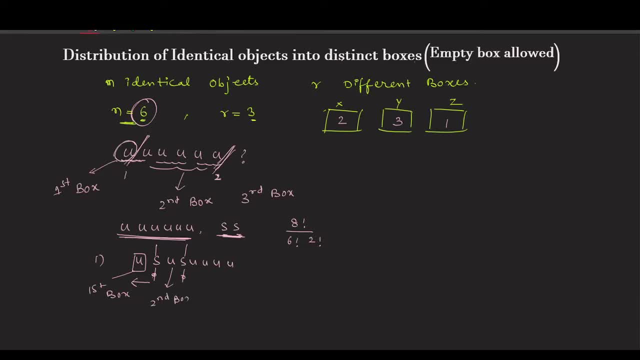 This will go to the second box. So I have an arrangement of u's and s and this will go to the third box. So one arrangement is giving what One distribution Right? So one arrangement is giving one distribution means how many distributions are possible. 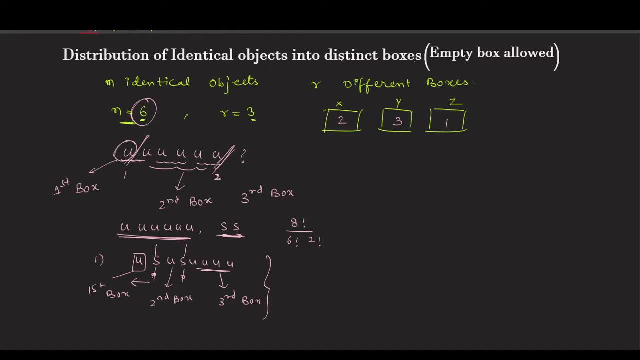 How many ways you can distribute the objects. Right, How many ways you can distribute the objects means how many arrangements are possible. So how many arrangements? the question for that question? the answer is: eight factorial by six factorial into two factorial. 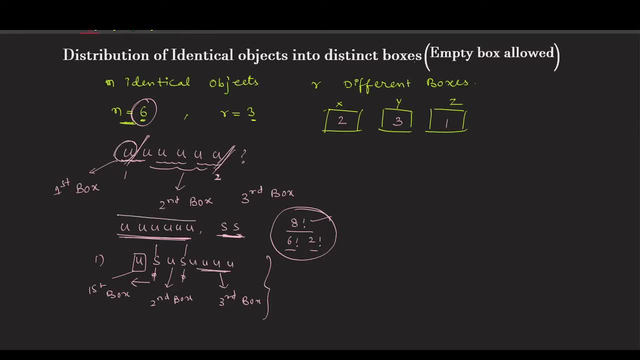 Now here the question is this: So whenever six identical objects given to you, you are taking six u's and you are taking two separation symbols only. Why we need two separation symbols? Because of we want three groups, you know. So here we have to divide into three groups to distribute into three boxes. 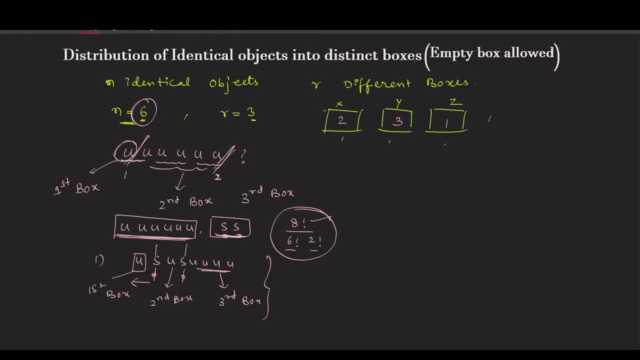 So we need only two separation symbols. For example, I have one more box extra here, t. One more box extra t box you have. Now I have to distribute this six u's into four boxes. I have to distribute this six u's into four boxes. 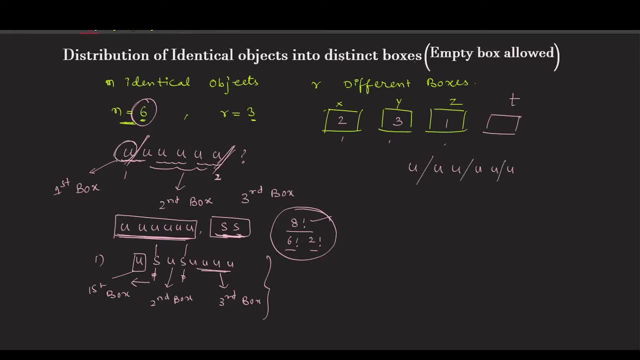 So I need three separation symbols. You see, here I need, like this, three separation symbols. Then this will go to the first box, These two u's will go to the second box, These two u's will go to the third box, and the last u will go to the fourth box. 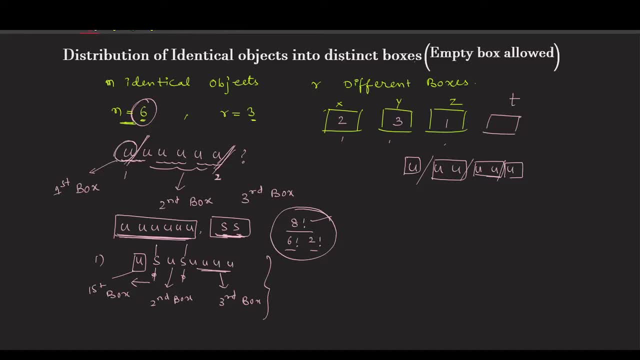 So what does it mean? So what does it mean? How many boxes are there? How many boxes are there? That many minus one will be the separation symbols. How many separation symbols we need is the number of boxes minus one. So your number of boxes are four. 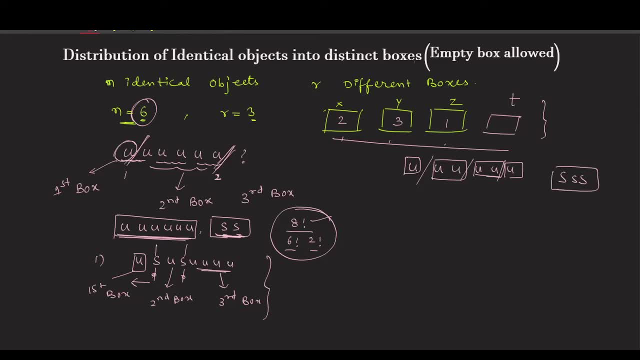 So separation symbols we need, how many? Three Means how many ways you can arrange six u's and three s, How many ways you can arrange Totally. here we have six plus three. Total nine letters are there. These nine letters can be arranged in nine factorial ways. 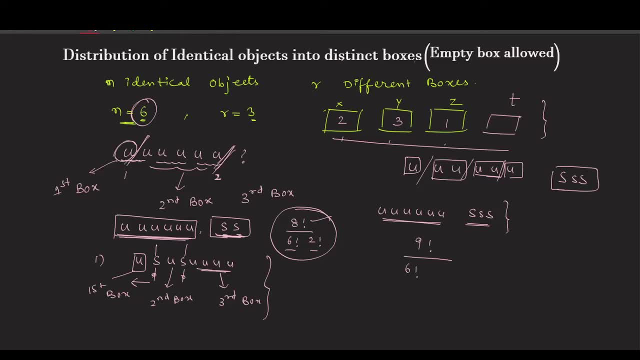 But among which we have six u's, so six factorial and three s, therefore three factorial, So nine factorial by six factorial into three factorial. This is the number of total number of arrangements. Now have I, as I told you, as I told you, each arrangement is one distribution. 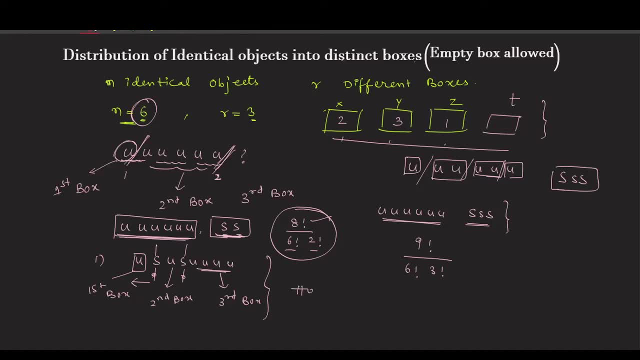 Each arrangement is one distribution. So if I ask you how many ways, If I ask you how many ways These, These objects can be distributed, How many ways these objects can be distributed, If I ask you like this, the question is similar to the number of arrangements, is nothing but. 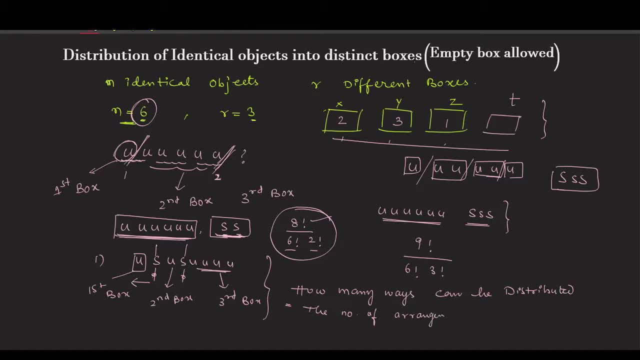 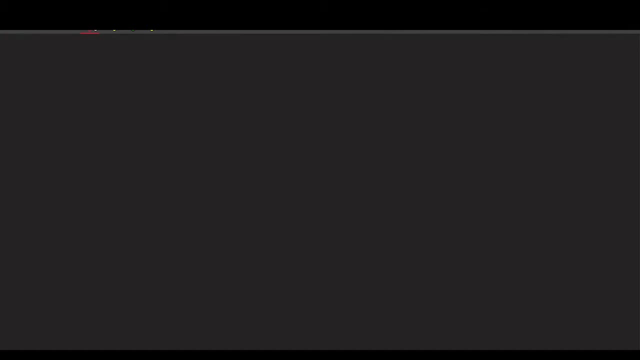 the number of arrangements of taking that six u's and two separation symbols if three boxes are there. So number of distributions is going to be number of arrangements. Now let us finalize the result, Now say you have what? once again, I will repeat the procedure: six, identical box six. 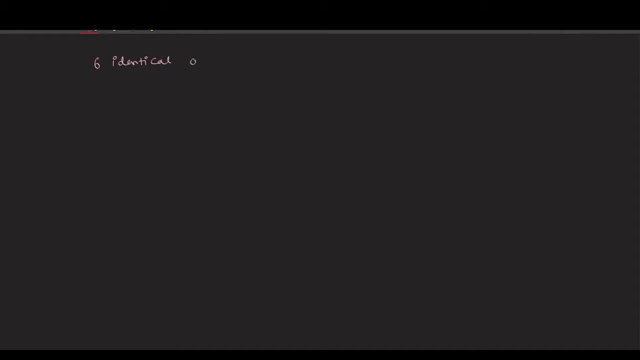 identical objects you have, six identical objects you have and three different boxes you want to distribute. Then what will be the answer we got? That is nothing but six u's and two s. how many ways you can arrange The final answer is eight. factorial. by what? 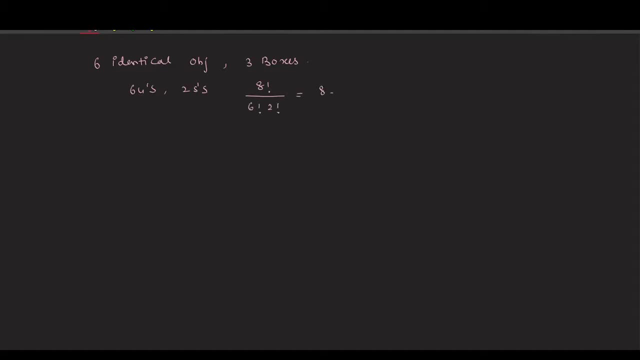 Six factorial into two factorial. Then you see, this is nothing but eight c two. This is nothing but eight c two. Now let us see the second one. what I told you is, if you have six identical, six identical objects you have, and you have four different boxes, then how many separation symbols we 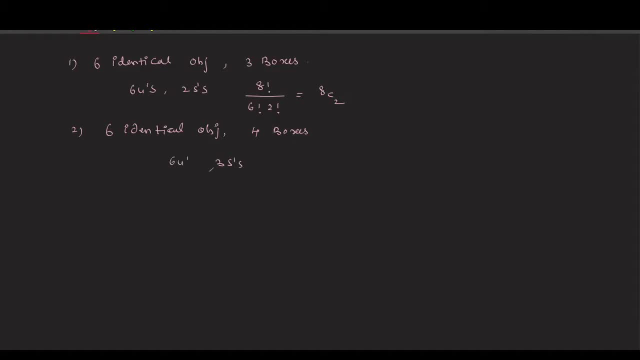 need Three s and six u's. How many ways you can arrange total number of letters? nine factorial divided by six u's are identical: six factorial and three s. this is three factorial, which is nothing but nine c three. Let us see one more so that we can finalize the formula. 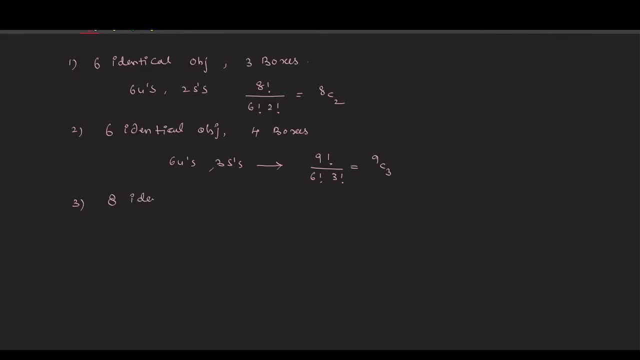 Let us suppose you have eight identical objects. Suppose you have eight identical objects and you have, let us say, five different boxes. You have five different boxes. Now, in this case, what we will do to distribute Eight identical objects means you can think of eight u's and how many separation symbols. 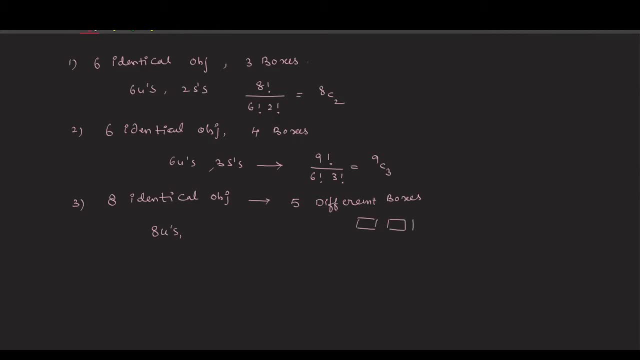 we need? See, we want to distribute into five different boxes. right, We want to distribute into five different boxes means how many separation symbols? you need Four separation symbols. yes, So four separation symbols. How many ways you can arrange eight u's four s totally twelve we have. so twelve factorial 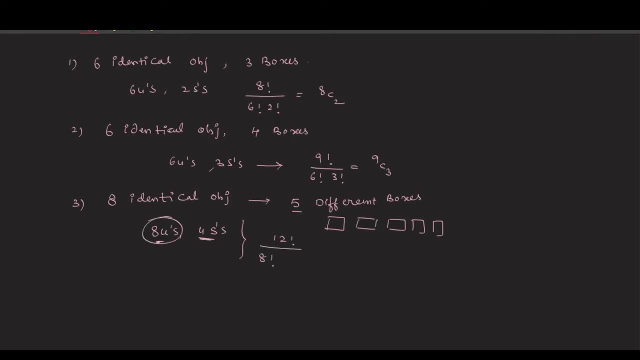 divided by eight. u's are identical, So we write eight u's, We write eight factorial. four s are identical, so we write four factorial, which is nothing but twelve c four. Now you observe here How you got this: two here, Two and three and this four. they are separation symbols. 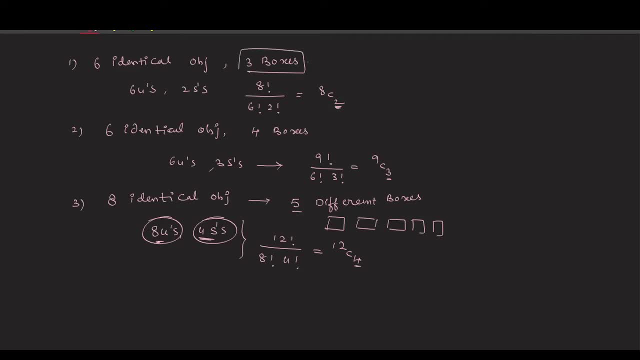 How you got that. Separation symbols is equals to number of boxes minus one, that is separation symbols. Four boxes minus one: that is separation symbols. Five different boxes minus one, that is separation symbol, which is nothing but this one. So if you have n identical objects, 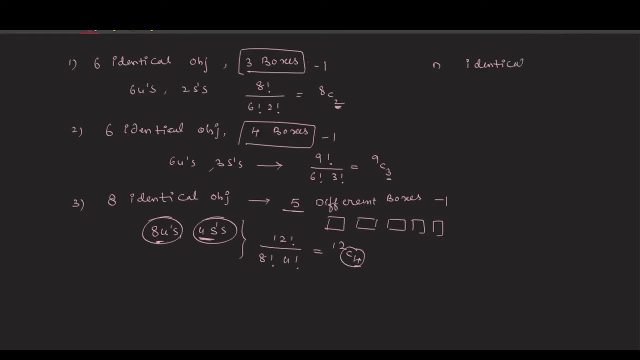 If you have n identical objects and you want to distribute into r different boxes, r different boxes, How many ways it can be done? right, Different boxes minus one will be your separation symbols. okay, So you will write c r minus one. 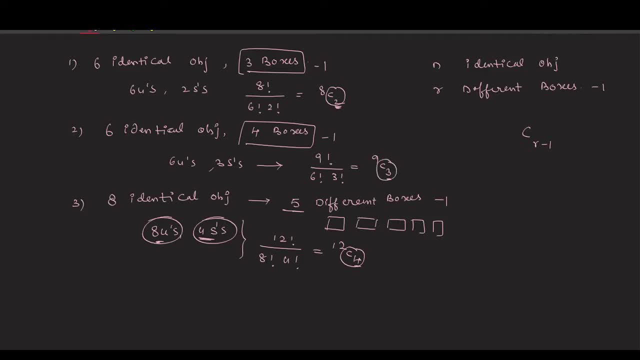 Can you see here c two? Can you see here c three? Can you see here c four? Four is separation symbol. three is separation symbol two, So r minus one. And how you got this number eight, How you got this. Six use plus separation symbols. six. use plus four separation symbols. sorry, separation. 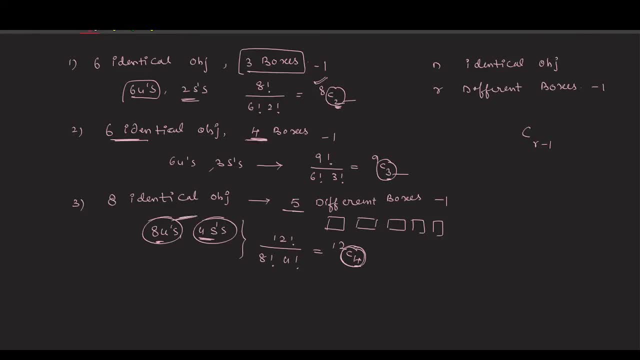 symbol is three, So four, six plus three, nine. Here we have eight use and four separation. eight plus four, twelve, So here we have r minus one. separation symbols and objects are n. So what you have to write here: n plus r minus one, c r minus one. 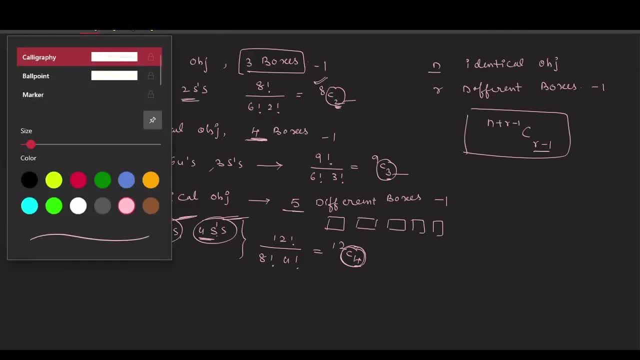 So the final conclusion is: The final conclusion is: N plus r minus one, c r minus one. So the final conclusion is: So the number of the number of ways of distributing, the number of ways of distributing n identical objects, n identical objects into r different boxes, into r different boxes, r into different. 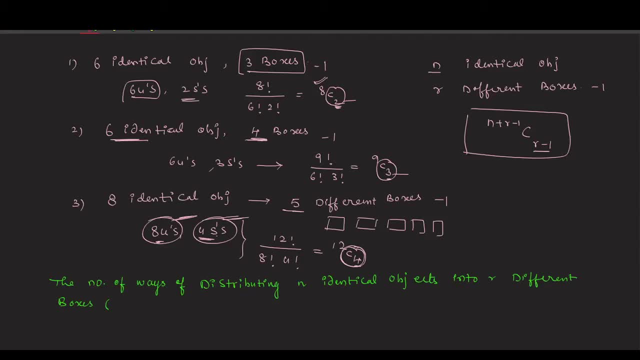 boxes where box can be empty. empty box is allowed. box can be empty. box may be empty. box may be empty. is what n plus r minus 1, c r minus 1, number of ways of distributing n identical objects into r different boxes where maybe a box can be empty. is what n. 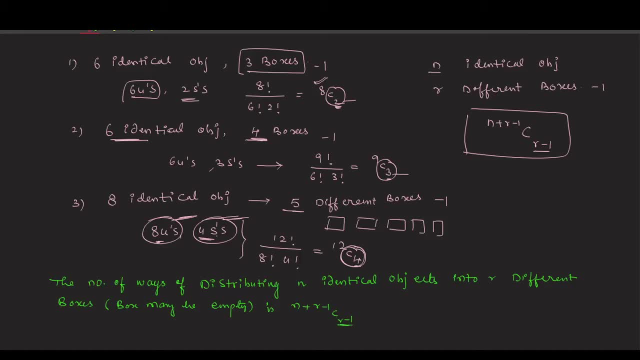 plus r minus 1, c r minus 1, keep in mind this: r minus 1, how you got number of boxes minus 1, number of boxes minus 1, right, and add the objects. how many are there n objects? 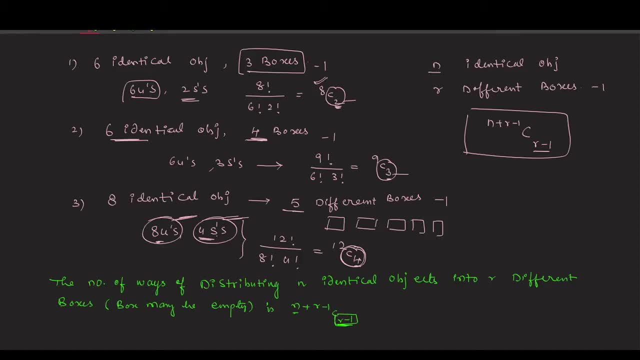 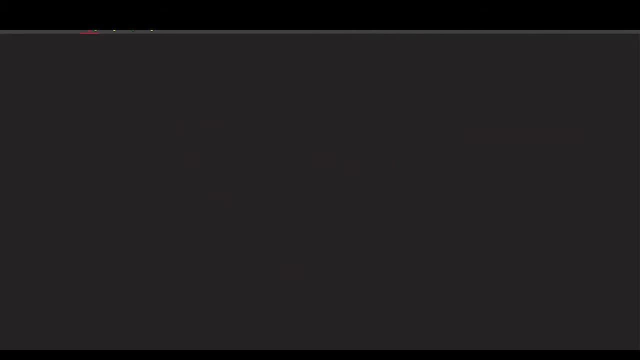 are there. so you add that n to that r minus 1, okay, Now let us see. for example, if I ask you how many ways, how many ways? 8 apples. so here we consider, all the apples are identical. 8 apples can be distributed, can be distributed. 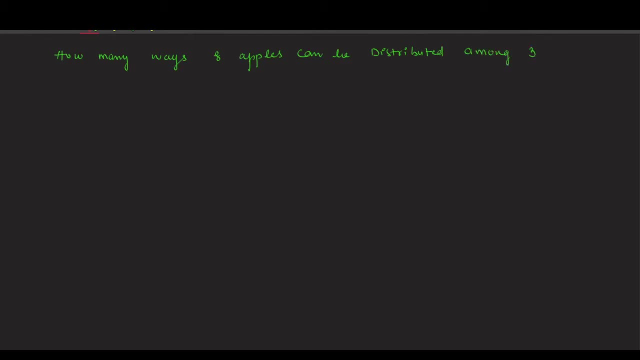 among 8 apples, 3 children. okay, so this is the question: how many ways? a simple, basic question. actually we will see some advanced questions later. how many ways 8 apples can be distributed to 3 children? so here, 3 children we will suppose as different. only there is no doubt. 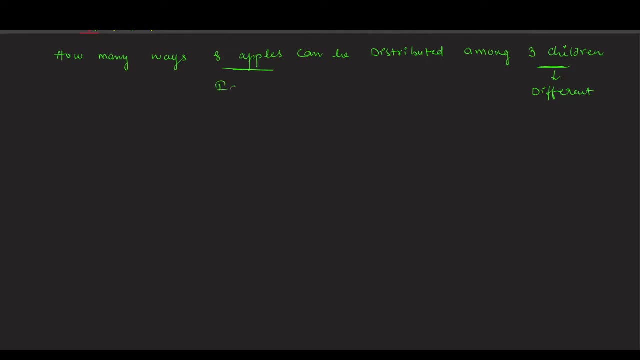 in that. and apples are identical, so identical into different right, so 8, and different is boxes. how many 3 boxes you can think of as a boxes? 8 apples into 3 boxes, nothing but 3 children. so how many separation symbols we need different boxes? 3 minus 1, so we 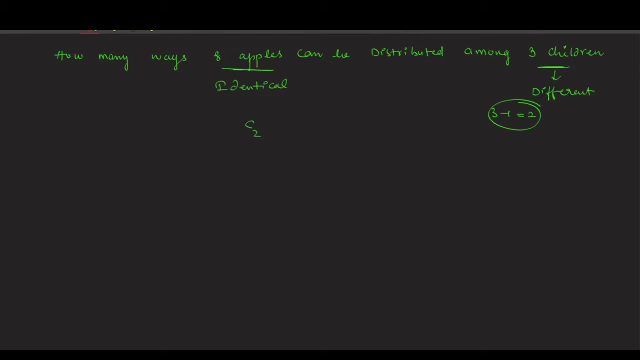 need 2 separation symbols, so we write c 2 and we add objects plus this separation symbols, 8 plus 2, c 2, which is 10, c 2, which is nothing. but you can calculate 10 into 9 in by 2, which. 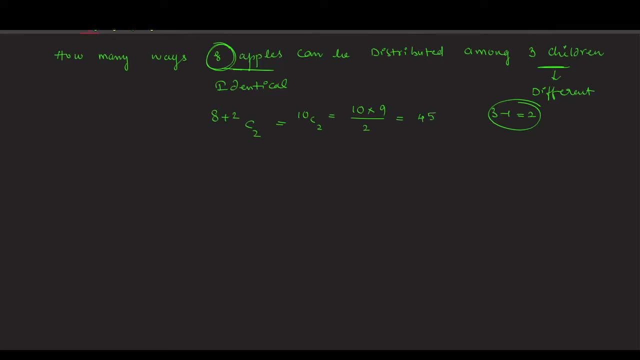 is 45 ways, So 8 apples can be distributed among 3 children in 45 ways. right? so if you know that rule, how we derive, it is very simple to remember the formula also. okay, if you want to distribute. 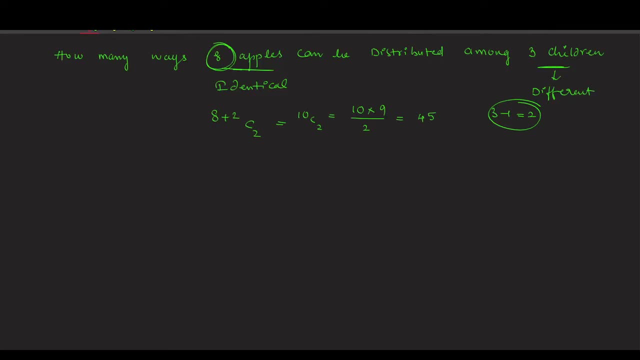 into 3 boxes, 3 different boxes. you have to take 2 separation symbols, so which gives you c 2, and that separation symbol should be added to how many objects are there? 8 objects, 8 plus 2 c 2.. 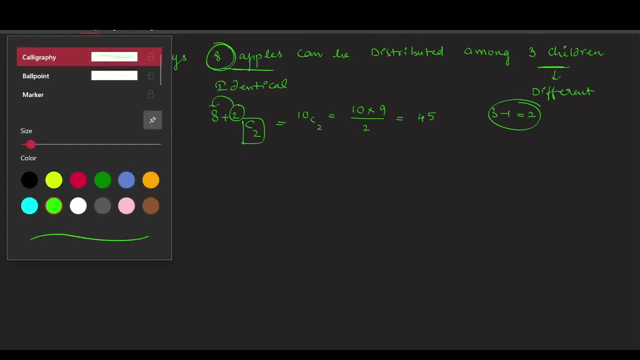 For example- I will ask a different question now. you see Question number 2,. for example: find the number of non-negative. find the number of non-negative integral solutions, number of non-negative integral solutions of the linear equation x plus y plus 2.. 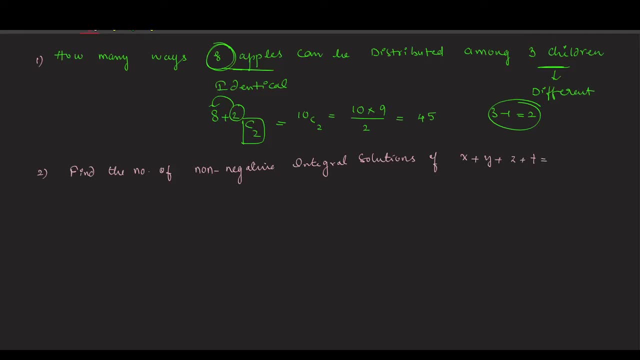 Okay, Okay, z plus t is equals to, let's say, 11. here we have to find out the number of non-negative integral solution means x value may be 0 or positive, y value also may be 0 or positive, z value may be 0 positive and t value may be 0 or positive, and the equation is: x plus y plus z plus t is equal. 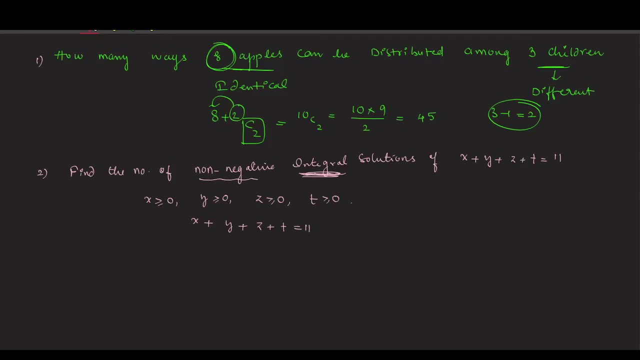 to 11 and number of integral solutions. we want integer solutions. okay, now say you have four boxes. okay, i give names to these boxes. i'll mark the first box by x, the second box by y, third box by z and fourth box by t. now can you tell me this? 11 means number of integral solution, means, if i put 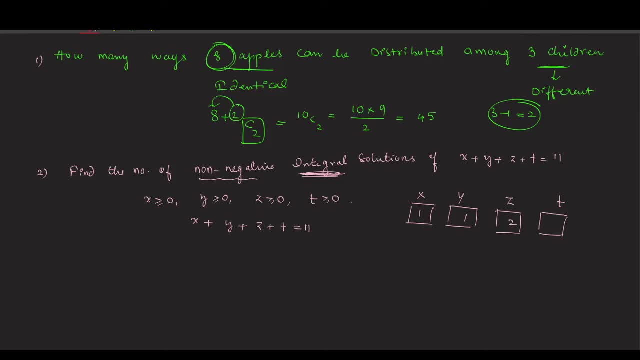 here one, here one, here two, so four plus how much i have to put the number here in the t box- four already gone, so seven. can you tell me the number of integral solutions we want to find out? you see, one x value, one y value, one z value, two t value. seven is nothing but distribution of this. 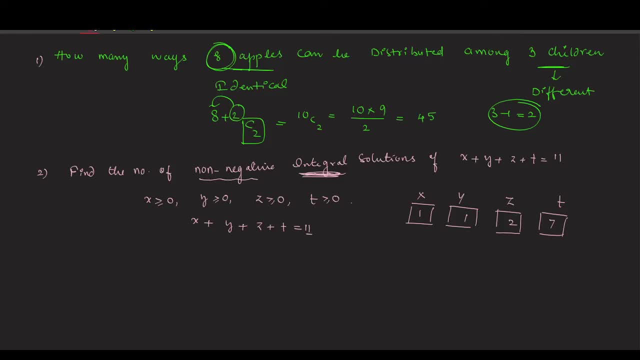 11. you can suppose this distribution of 11 identical objects into four boxes: one one, two, seven or zero, zero, one, ten or maybe zero five, four, nine, two. this is also one way of arrangement, right, one way of distribution. so what is the question? indirectly, how many ways you can arrange. 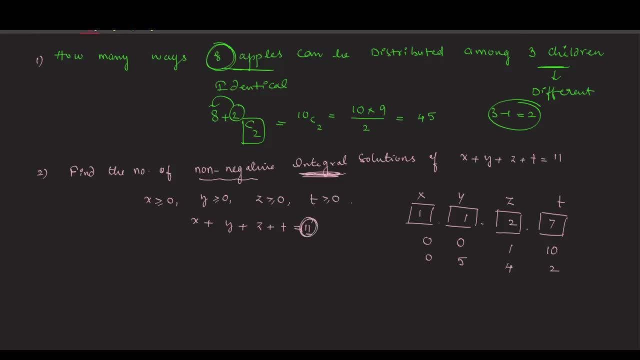 11 objects identical, which are identical, 11 identical objects into four different boxes right, different boxes because of x value, y, z, t, different variables. we have so different boxes, you can suppose, and 11 means two ones, three ones, four ones, right, seven means seven ones, two ones, one, one one.